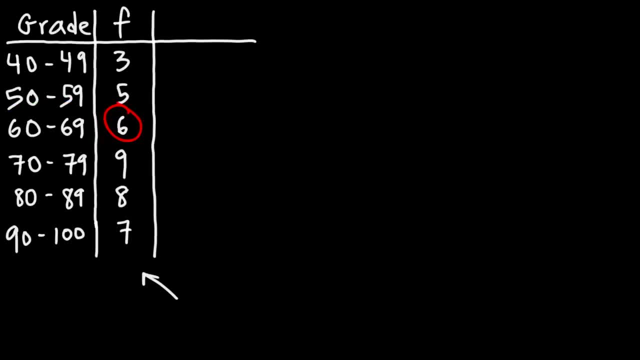 students who got a D on the exam, eight students who had a score between 80 and 89. So, with this data, how can we calculate the average test score of the students in this class? Now it's important to understand that we cannot compute an exact mean for the. 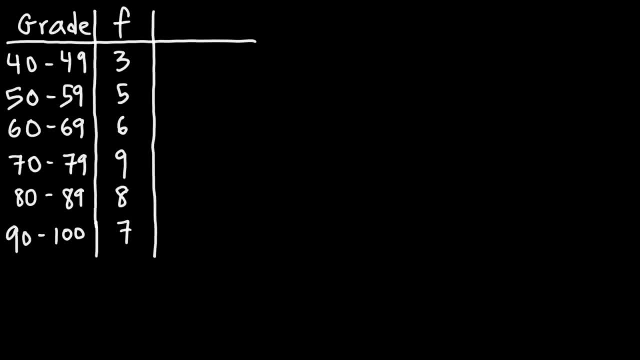 grades in this class. And the reason why that's the case is because we just don't know the individual data values in the data set, So therefore we can estimate the mean. Now we know that the mean is basically the sum of all the data values. 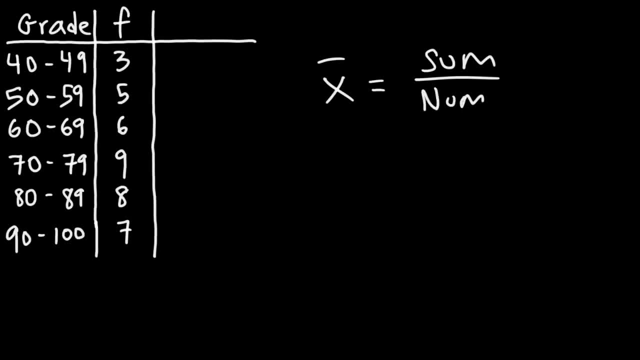 divided by the number of data items in the set. But for a group frequency table the mean is going to be something similar, but that equation will be modified a bit. It's going to be the sum of the product of the frequency values times the midpoint, because we can't really use an 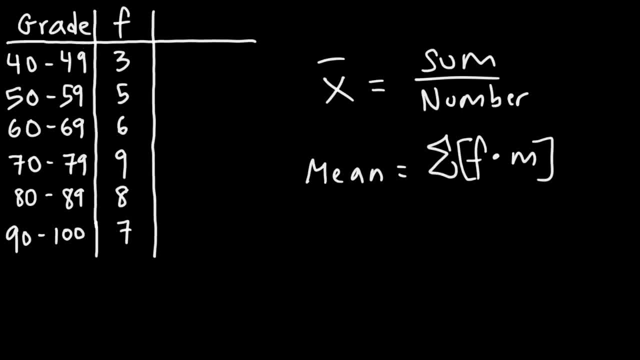 individual score here, since we have an interval, So the best ideal individual score would be the midpoint of each grade interval. So it's going to be the sum of the frequency times, the midpoint divided by the sum of the frequency values, And so that's the formula that we need to use in. 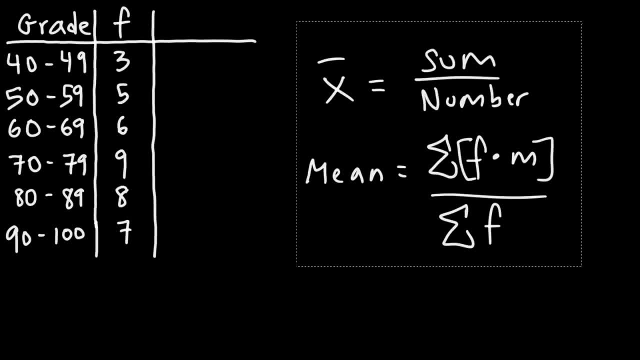 order to calculate the mean. So let's take this one step at a time. Let's calculate the midpoint values first. The midpoint is going to be the sum of the lower boundary of the interval plus the upper boundary of the interval, divided by 2.. So in the grade interval of 40 to 49, the lower 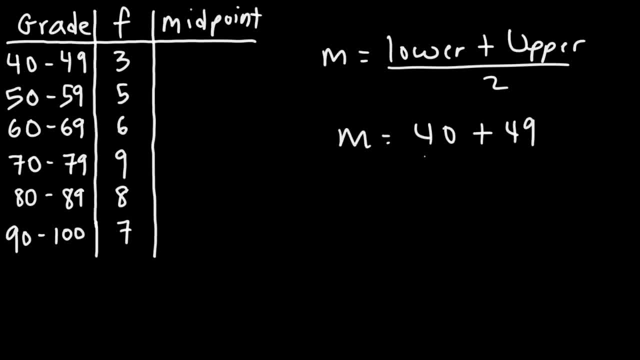 boundary will be 40.. The upper boundary is 49 divided by 2.. So we get 89 divided by 2, which is 44.5.. So that's the midpoint for this interval. Now let's do the same for the next one. So the second midpoint is going to be 50 plus 50. 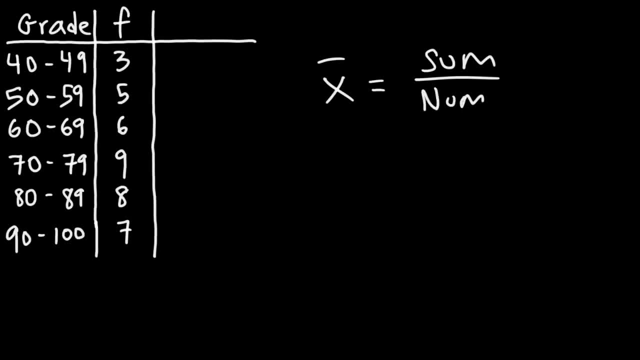 divided by the number of data items in the set. But for a group frequency table the mean is going to be something similar, but that equation will be modified a bit. It's going to be the sum of the product of the frequency values times the midpoint, because we can't really use an 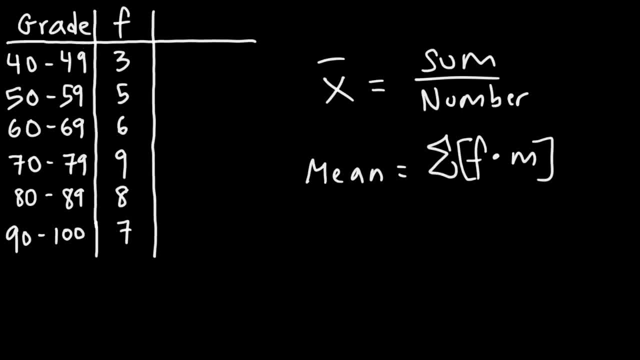 individual score here, since we have an interval, So the best ideal individual score would be the midpoint of each grade interval. So it's going to be the sum of the frequency times, the midpoint divided by the sum of the frequency values, And so that's the formula that we need to use in. 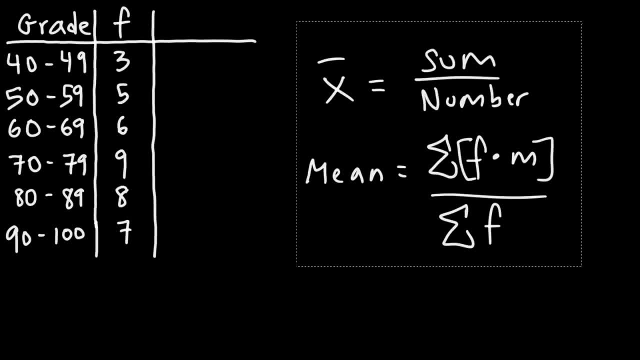 order to calculate the mean. So let's take this one step at a time. Let's calculate the midpoint values first. The midpoint is going to be the sum of the lower boundary of the interval plus the upper boundary of the interval, divided by 2.. So in the grade interval of 40 to 49, the lower 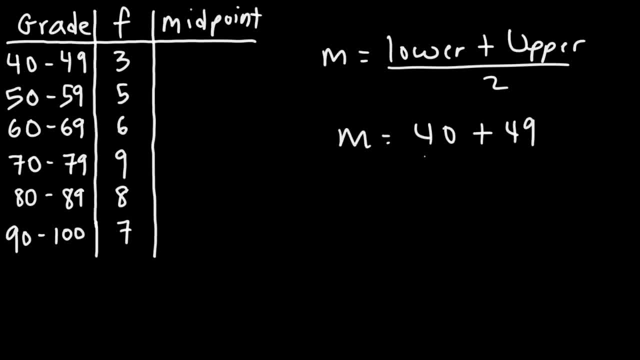 boundary will be 40,. the upper boundary is 49 divided by 2.. So we get 89 divided by 2, which is 44.5.. So that's the midpoint for this interval. Now let's do the same for the next one. So the second midpoint is going to be 50 plus 50. 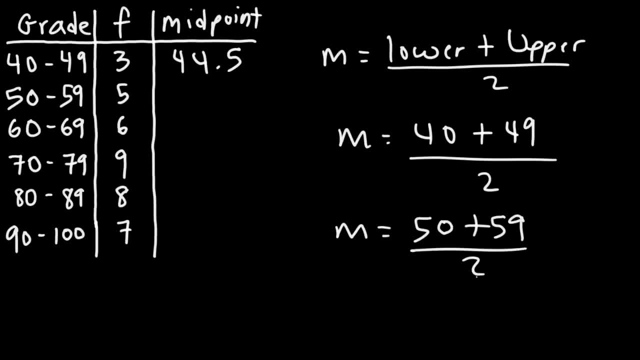 which is 59 divided by 2.. And so that's 109 divided by 2, which is 54.5.. At this point we can see a pattern. The next one is going to be 64.5, and then 74.5, and 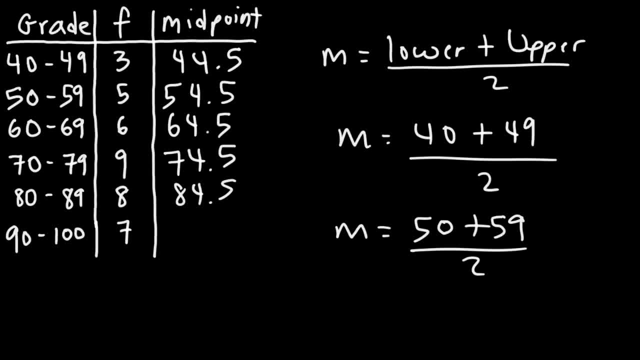 then 84.5.. The last one is different. So it's 90 plus 100, which is 190 divided by 2. This is going to be 95.. Now our next step is to take the sum of the frequency column. So this will give us: 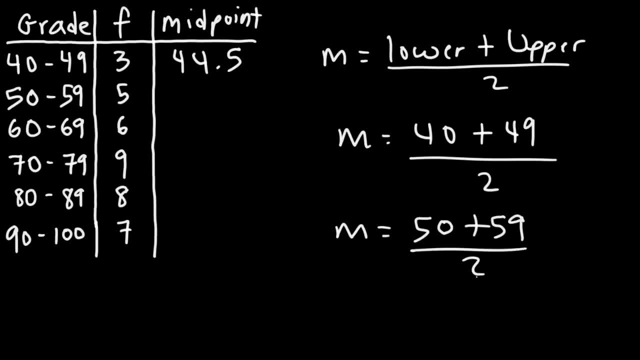 59 divided by 2.. And so that's 109 divided by 2, which is 54.5.. At this point we can see a pattern. The next one is going to be 64.5, and then 74.5,, and then 84.5.. 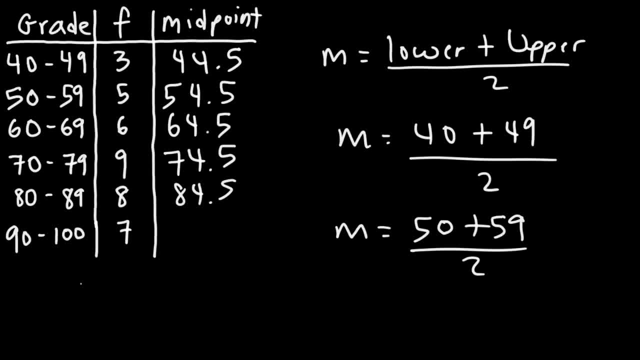 The last one is different, So it's 90 plus 100, which is 190, divided by 2. This is going to be 95.. Now our next step is to take the sum of the frequency column. So this will give us this particular value which will help us to calculate the mean. 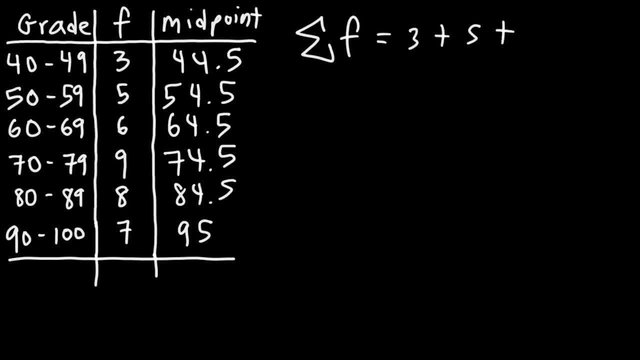 So it's going to be 3 plus 5 plus 6 plus 9 plus 8 plus 7.. So this tells us that we have a sum of the frequency column And this tells us how many students are in the class, And so there's a total of 38 students in this class. 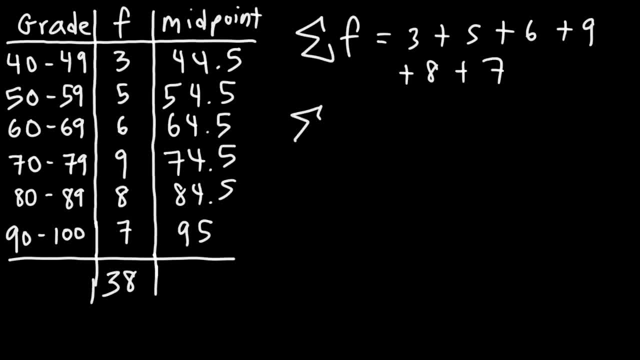 Now the next thing we need to calculate is the sum of the frequency times, the midpoint values. So what we're going to do is multiply these two. Now it might be easier to basically make an extra column And then sum up those values. 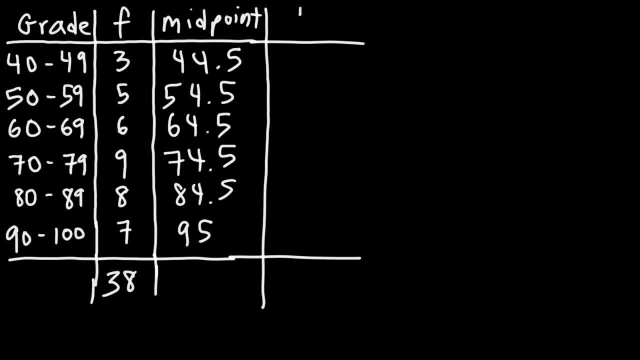 Okay, that line is not straight, So let's call this F times M. So what we're going to do is multiply the frequency by the midpoint, So 3 times 44.5.. And that's going to be 133.5.. 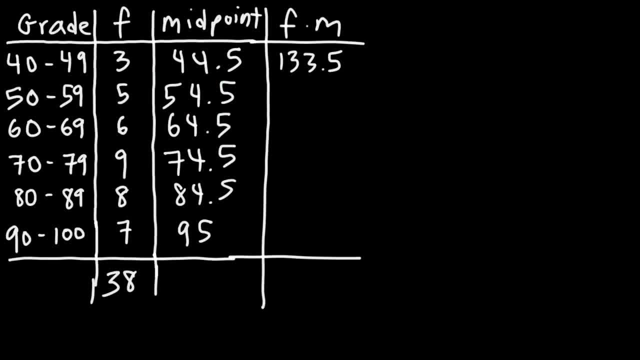 And then multiply these two values, So that's 5.5.. 5 times 54.5,, which is 272.5.. And then 6 times 64.5.. So that's going to be 387.. And then 9 times 74.5,, which is 670.5.. 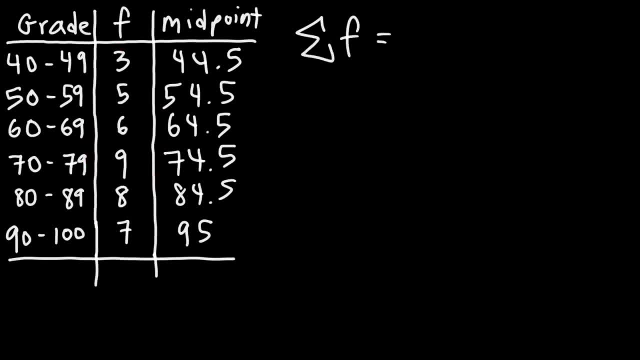 this particular value which will help us to calculate the mean. So it's going to be 3 plus 5 plus 6 plus 9 plus 8 plus 7.. So this tells us how many students are in the class, and so there's a total of 38 students in. 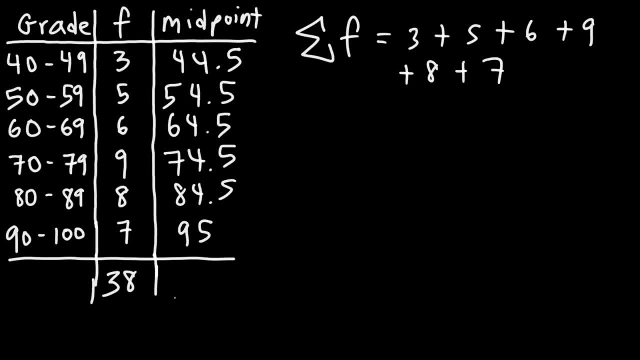 this class. Now the next thing we need to calculate is the sum of the frequency times, the midpoint values. So we're going to do is multiply these two. Now it might be easier to basically make an extra column And then sum up those values. 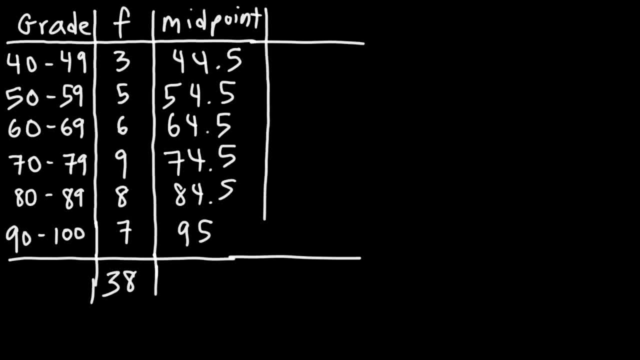 Ok, that line is not straight, So let's call this f times m. So what we're going to do is multiply the frequency by the midpoint, So 3 times 44.5, and that's going to be 133.5, and then multiply these two values. 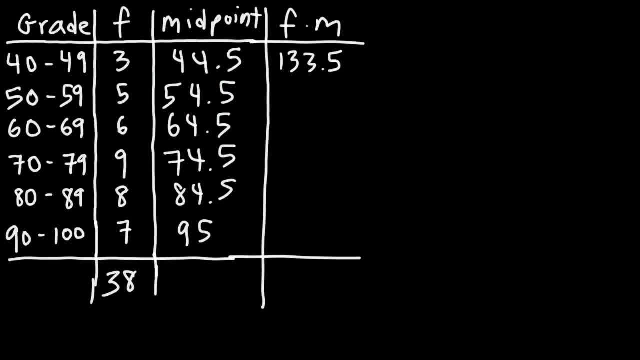 So that's 3 times 44.5.. 5 times 54.5,, which is 272.5.. And then 6 times 64.5.. So that's going to be 387, and then 9 times 74.5,, which is 670.5.. And then 8 times. 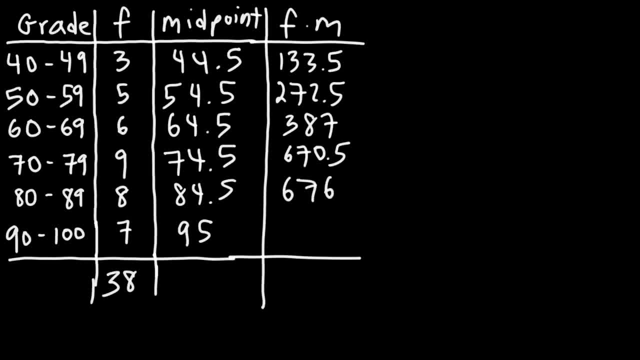 84.5, that's 676.. And finally, 7 times 95 is 665.. Now let's take the sum of this column, So go ahead and add those numbers using the calculator, So the total that I have is 2,804.5.. 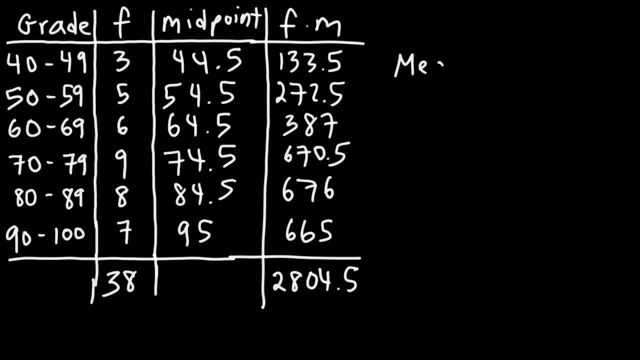 So now we can calculate the mean. The mean is going to be the sum of the FM values divided by the sum of the frequency values. So this right here, basically all of this, correlates to this number. So that's 2,804.5.. 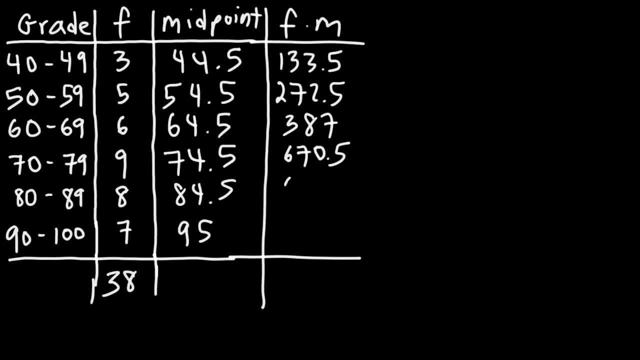 And then 8 times 84.5.. That's 676.. And finally, 7.5.. 7 times 95 is 665.. Now let's take the sum of this column. So go ahead and add those numbers using the calculator. 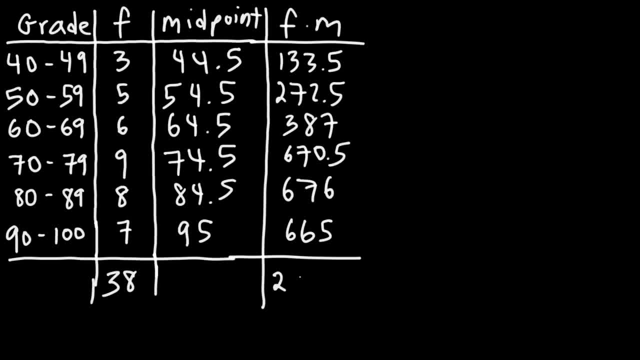 So the total that I have is 2804.5.. So now we can calculate the mean. The mean is going to be the sum of the FM values divided by the sum of the frequency values. So this right here, basically all of this. 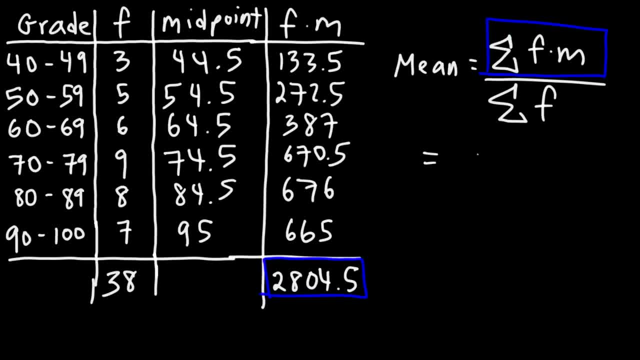 correlates to this number, So that's 2804.5.. And then divided by the sum of the frequency values which we have here, And that's 38.. Now, before we divide it, where do you think the mean is going to be? 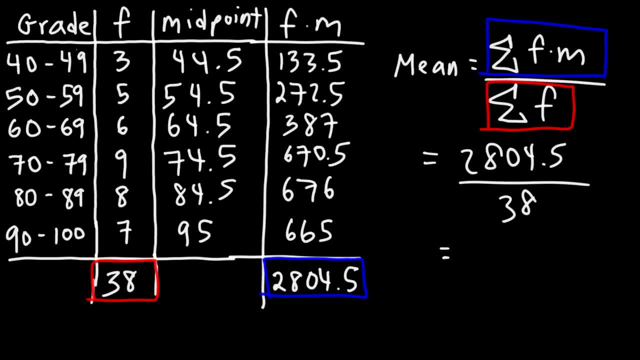 In which interval Will it be? in this interval, This one, This one, Which one? Notice that the highest frequency occurs here, So chances are the mean is going to be between 70 and 79. Because most students scored in that range. 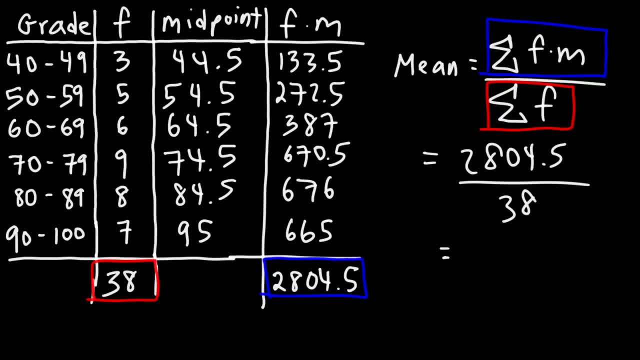 So if we take 2804.5, divided by 38,, this gives us a mean value of 73.8.. And that makes sense, since most students they had a C on the test. Now here is another question for you. 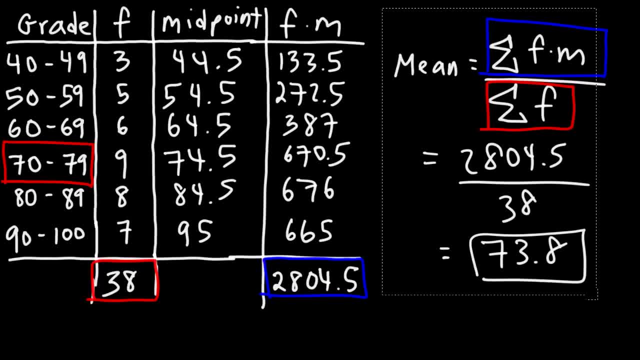 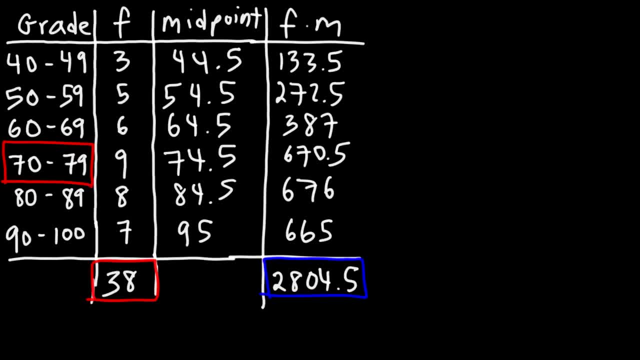 In which interval can the median and the mode be located? in What would you say? Now, the mode occurs where the frequency is the highest. So the frequency is the highest in this interval. So the mode exists between 70 and 79.. 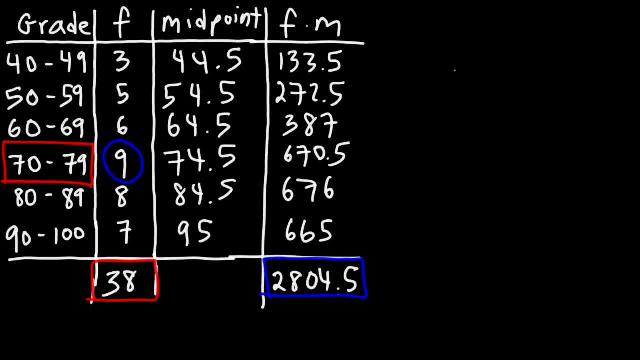 Now, what about the median? In order to figure that out, we need another column. So we're going to call this cumulative frequency. We're going to start with this number 3.. And then we're going to add 5 and 3 together. 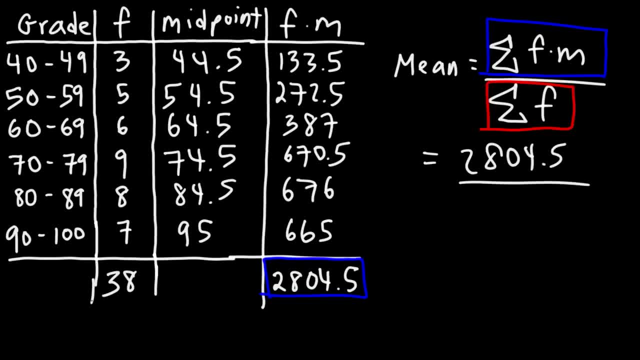 And then divided by the sum of the frequency values which we have here, And that's 38.. Now, before we divide it, where do you think the mean is going to be? In which interval Will it be? in this interval, this one, this one, which one? 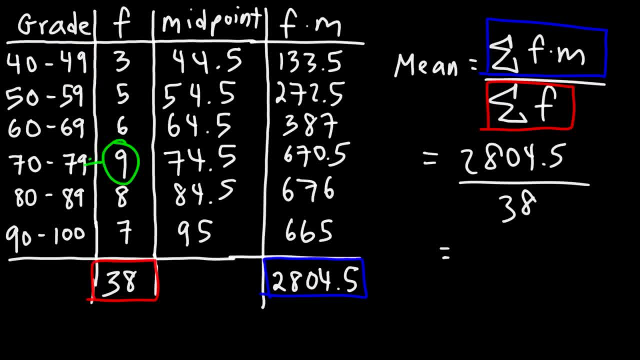 Notice that the highest frequency occurs here. So chances are the mean is going to be between 70 and 79. Because most students scored in that range. So if we take 2,804.5, divided by 38,, this gives us a mean value of 73.8.. 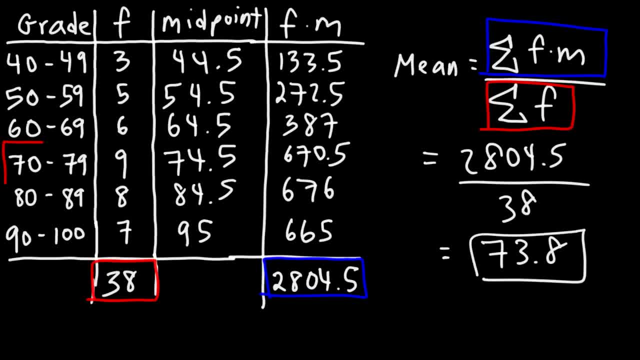 And that makes sense, since most students they had a C on the test. Now here is another question for you: In which interval can the median and the mode be located in? What would you say? Now, the mode occurs where the frequency is the highest. 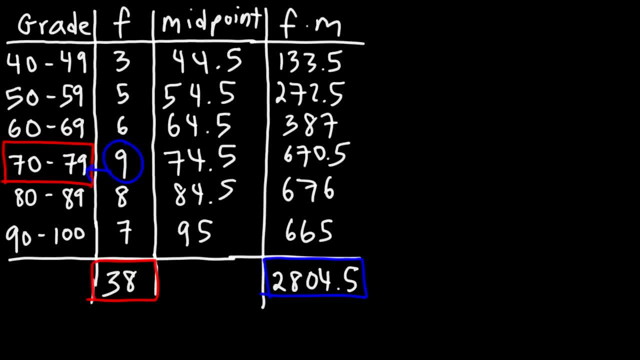 And the frequency is the highest. See, it's the highest in this interval. So the mode exists between 70 and 79. Now what about the median? In order to figure that out, we need another column. So we're going to call this cumulative frequency. 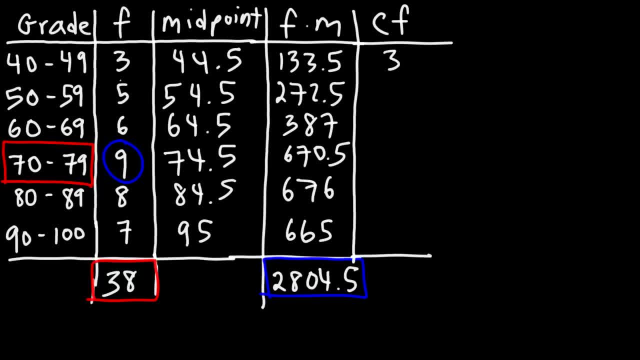 We're going to start with this number 3.. And then we're going to add 5 and 3 together, which will give us 8. Then we're going to take this number, add 6 to it. That's going to be 14.. 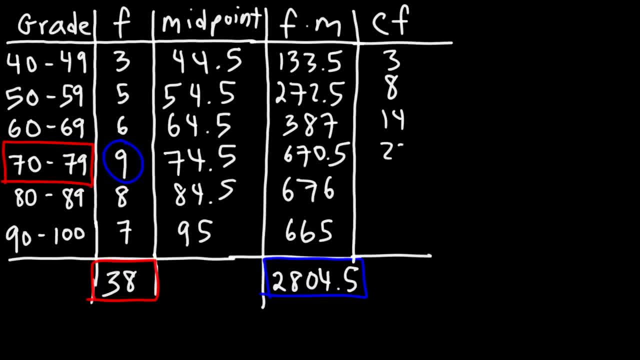 And then we're going to add 9 to 14, which gives us 23.. And then 23 plus 8 is 31.. And then 31 plus 7 is 38. So we get this number Because there are 38 students. 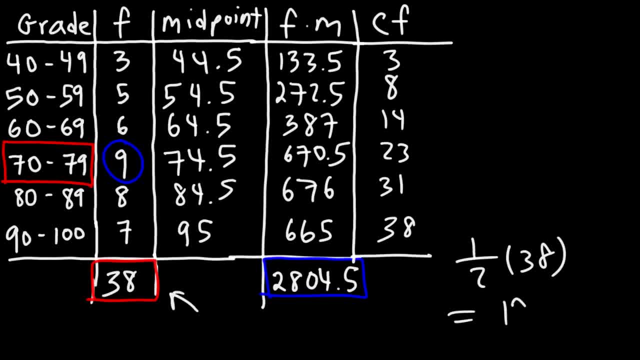 And half of 38 is 19.. So the middle number is basically the median. 19 is somewhere between 14 and 23.. So after 14, we're going to be done with this interval. 23 is in this interval between 70 and 79.. 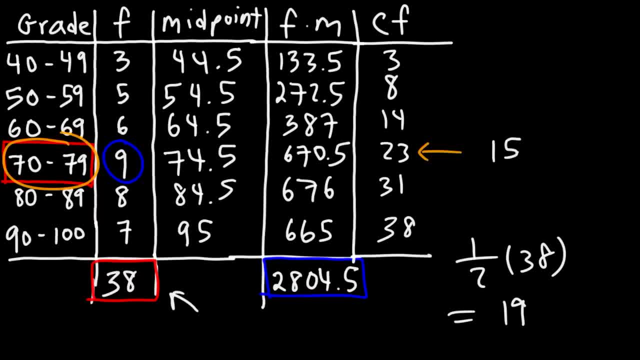 That interval starts with the number 15 and it ends in 23. And so 20 is in that interval. So the median is somewhere between 70 and 79 as well. Now let's work on another example for the sake of practice. 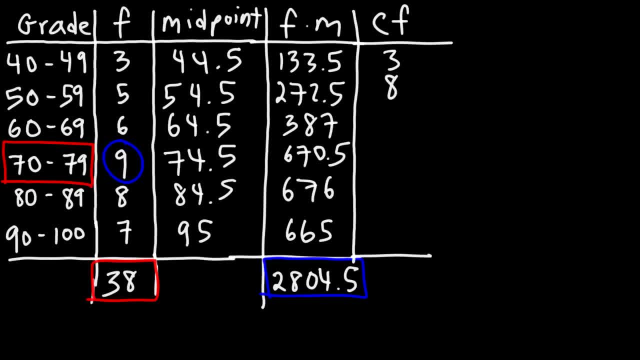 which will give us 8.. Then we're going to take this number, add 6 to it, That's going to be 14.. And then we're going to add 9 to 14, which gives us 23.. And then 23 plus 8 is 31.. 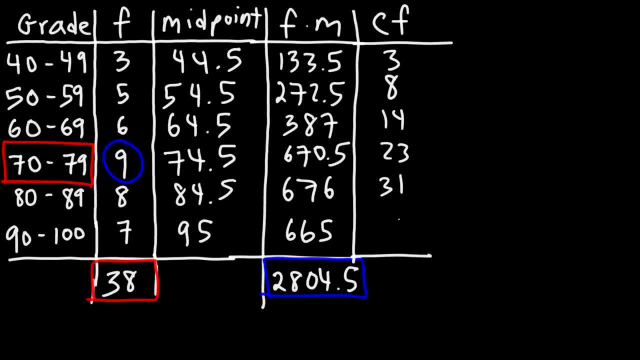 And then 31 plus 7 is 38. So we get this number Because there are 38 students And half of 38 is 19.. So the middle number is basically the median. 19 is somewhere between 14 and 24.. 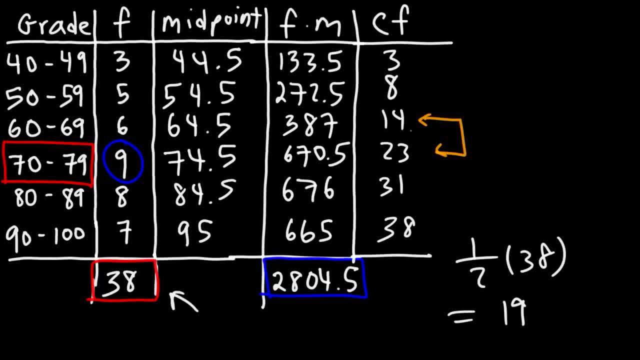 Between 14 and 23.. So after 14, we're going to be done with this interval. 23 is in this interval Between 70 and 79. That interval starts with the number 15 and it ends in 23.. 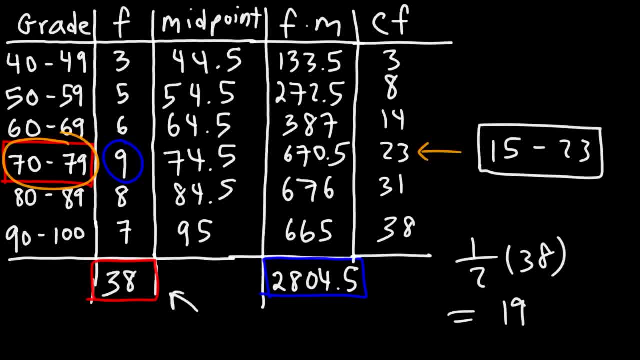 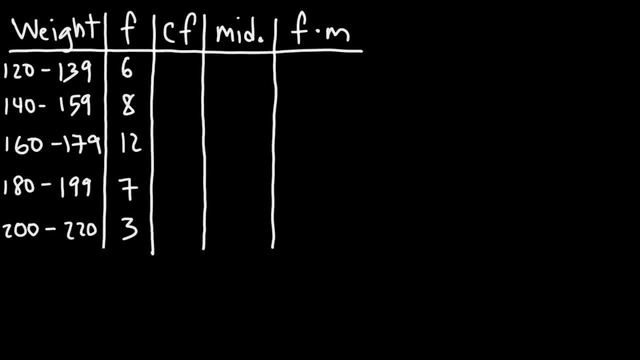 And so 20 is in that interval. So the median is somewhere between 70 and 79 as well. Now let's work on another example For the sake of practice. So here we have the weights of different students in a class, And what I want you to do is: 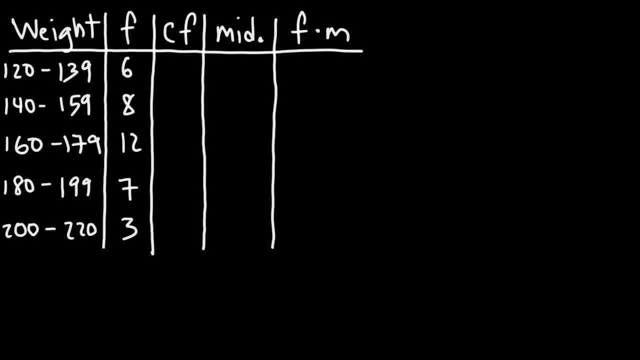 I want you to use this group data to calculate the mean and determine which interval contains the median and the mode. So go ahead and work on this example. So let's begin by calculating the cumulative frequency. So this is going to be 6.. 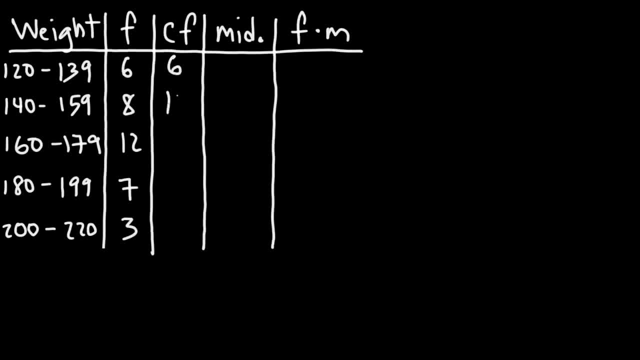 6 plus 8 is 14.. And then 14 plus 12 is 26.. 26 plus 7 is 33.. And 33 plus 3 is 36.. And if we basically take the sum of the frequency values, 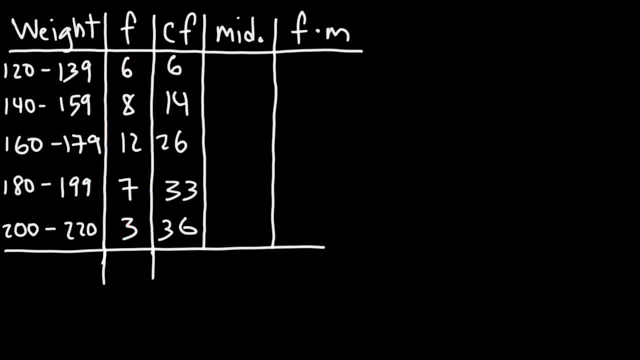 that should give us 36 as well, Which we can put down here. Now let's determine the midpoint values. So it's going to be the upper boundary plus the lower boundary divided by 2. Or vice versa. So the upper boundary is 139.. 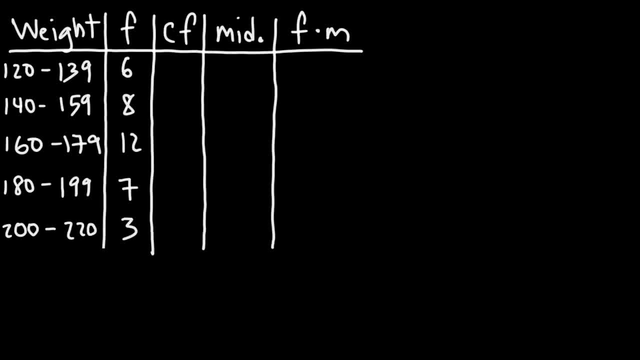 So here we have the weights of different students in a class, And what I want you to do is I want you to use this group data to calculate the mean and determine which interval contains the median and the mode. So go ahead and work on this example. 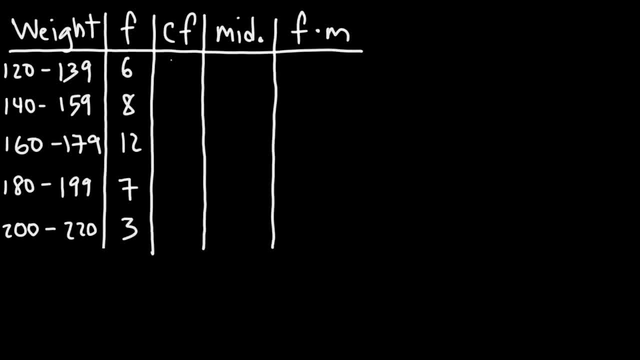 So let's begin by calculating the cumulative frequency. So this is going to be 6.. 6 plus 8 is 14.. And then 14 plus 12 is 26.. 26 plus 7 is 33.. And 33 plus 3 is 36.. 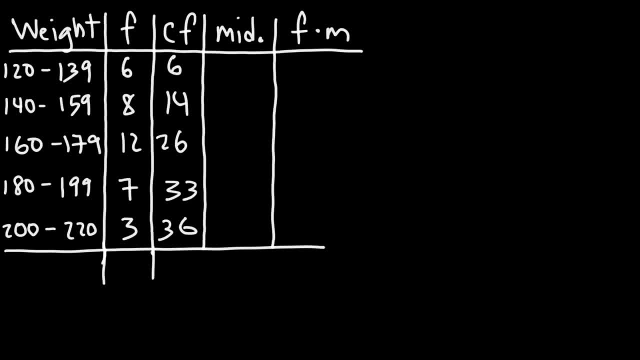 And if we basically take the sum of the frequency values, that should give us 36 as well, which we can put down here. Now let's determine the midpoint values. Okay, So it's going to be the upper boundary plus the lower boundary divided by 2, or vice versa. 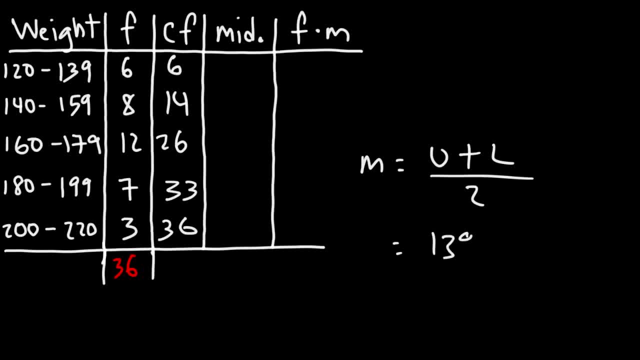 So the upper boundary is 139.. The lower boundary is 120 divided by 2.. So that's 259 divided by 2.. So the midpoint for the first interval is 129.5.. Now let's do the same for the second interval. 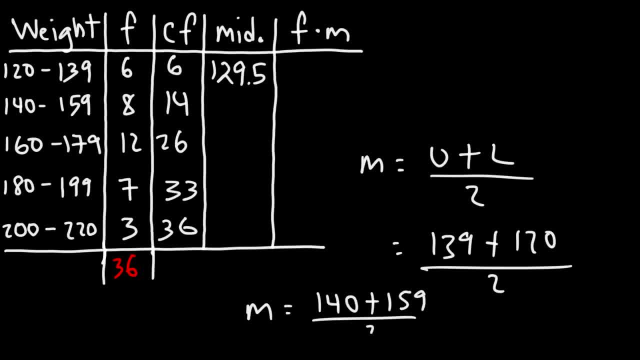 So let's add 140.. Let's add 140.. And 159.. And then divide by 2.. And so this is going to be 149.5.. So we can see that the midpoint is increasing by 20.. So the next one is going to be 169.5 and 189.5. 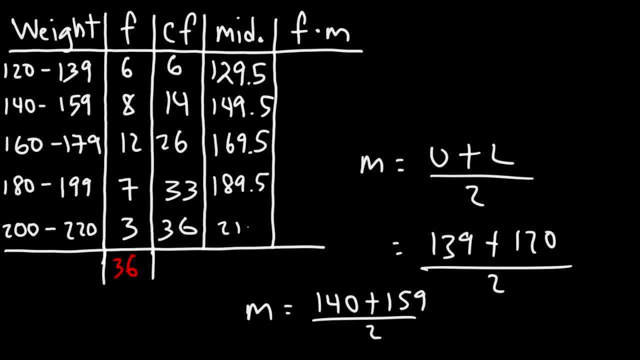 Now the midpoint between 200 and 220 is 210.. If you add these two, you're going to get 420.. 420 divided by 2 is 210.. Now let's take the frequency and multiply it by the midpoint. 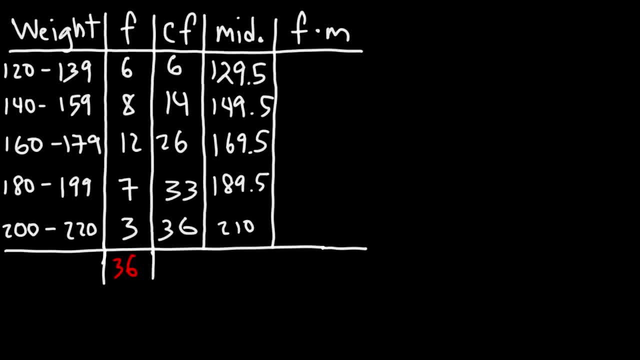 So 6 times 129.5, that's 777.. If we multiply 8 by 149.5, that's 1196.. And then 12 times 169.5.. This is going to be 2034.. And then 7 times 189.5.. 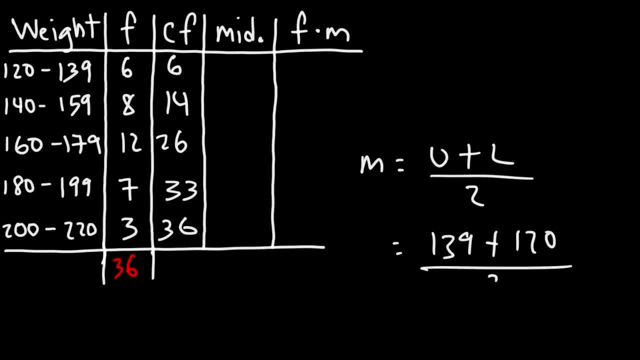 The lower boundary is 120 divided by 2.. So that's 259 divided by 2.. So the midpoint for the first interval is 129.5.. Now let's do the same for the second interval. So let's add 140 and 159. 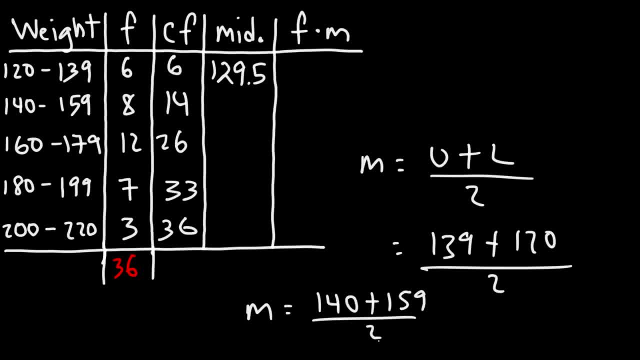 and then divide by 2., And so this is going to be 149.5.. So we can see that the midpoint is increasing by 20.. So the next one is going to be 169.5 and 189.5.. Now the midpoint between 200 and 220 is 210. 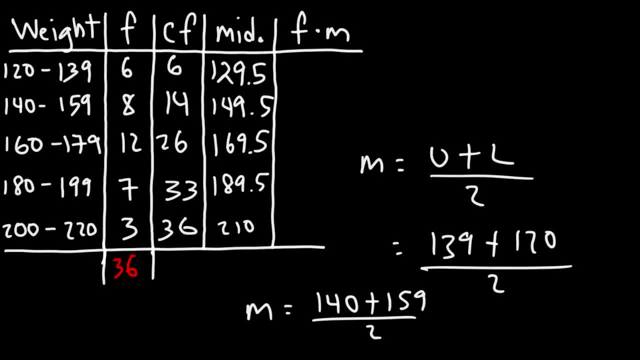 If you add these two, you're going to get 420.. 420 divided by 2 is 210.. Now let's take the frequency and multiply by the midpoint. So 6 times 129.5, that's 777.. If we multiply 8, 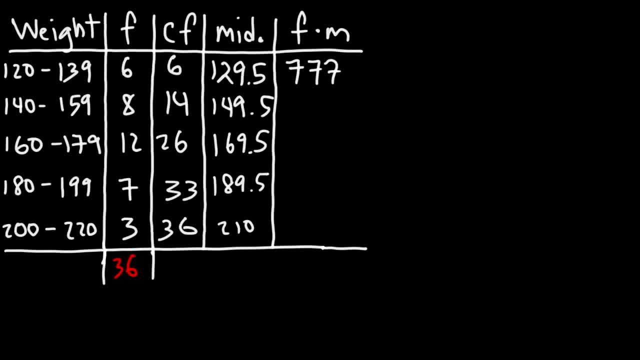 by 149.5, that's 1196.. And then 12 times 169.5, this is going to be 2034.. And then 7 times 189.5, that's 1326.5.. And then 3 times 210. 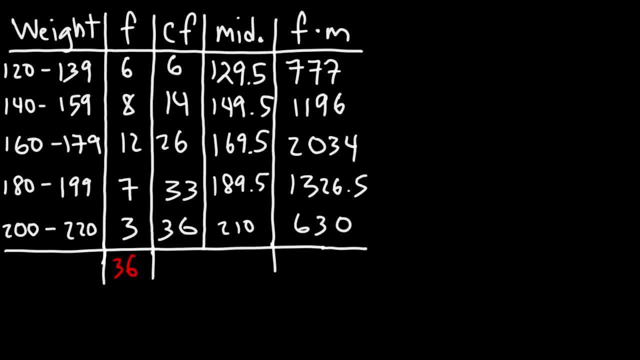 is 630.. So now let's take the sum of this column. So the sum is going to be- let's use a different color- 5963.5.. So at this point we can calculate the mean. So it's the sum of the frequency. 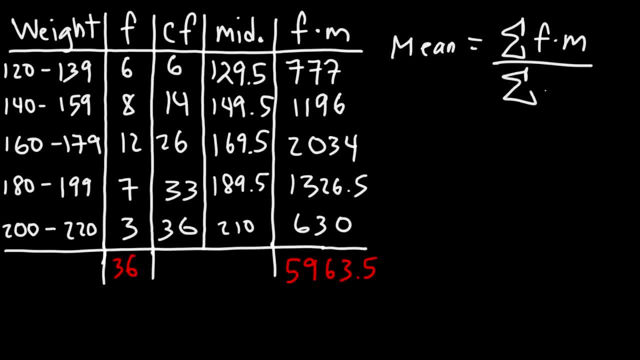 times the midpoint values divided by the sum of the frequency values. So we have this already, that's 5963.5.. And the sum of the frequency values is 36.. Now, before we calculate the mean, which interval do you think the mean is going to be? 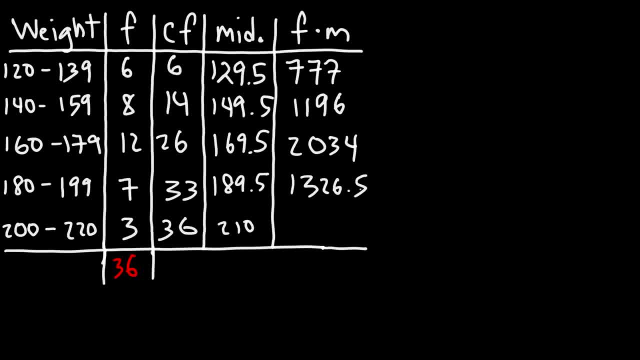 That's 1326.5.. And then 3 times 210 is 630.. So now let's take the sum of this column. So the sum is going to be- let's use a different color- 5,963.5.. 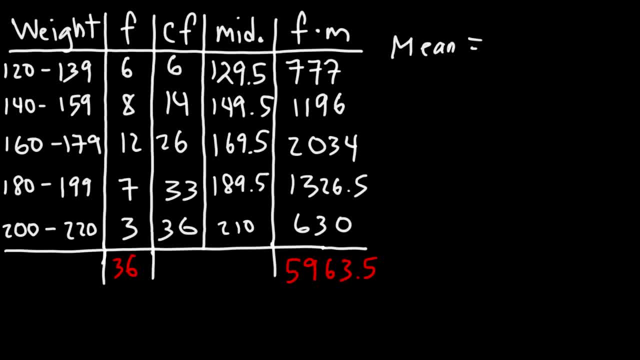 So at this point we can calculate the mean. So it's the sum of the frequency times, the midpoint values, divided by the sum of the frequency values. So we have this already. That's 5,963.5.. And the sum of the frequency values is 36.. 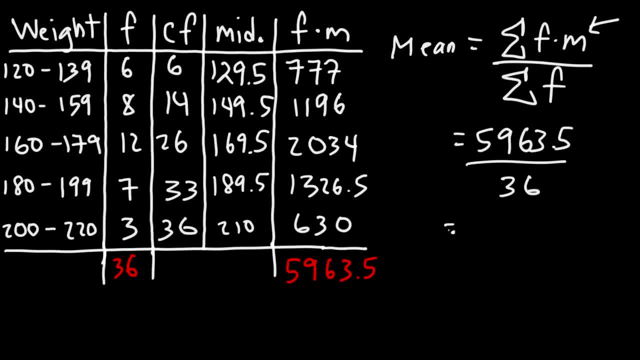 Now, before we calculate the mean, which interval do you think the mean is going to be? Now, most of the numbers are between 160 and 179. And the left side of the data is heavier than the right side of the data. 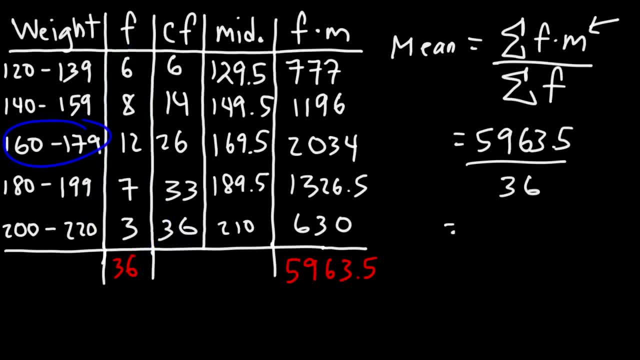 So it's either going to be in this interval or, in this interval, one of those two. So if we take 5963.5 divided by 36, that's going to give us 165.7 approximately. So that's the mean which turns out to be in this interval. 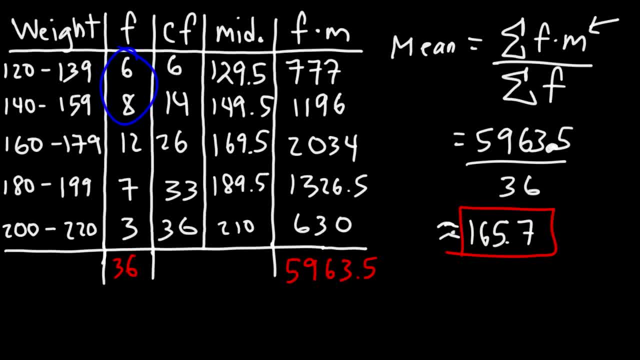 But notice that it's closer to 160 than it is to 179.. And this is due to the fact that the left side of the data is heavier than the right side of the data. Now, which interval contains the median and the median? 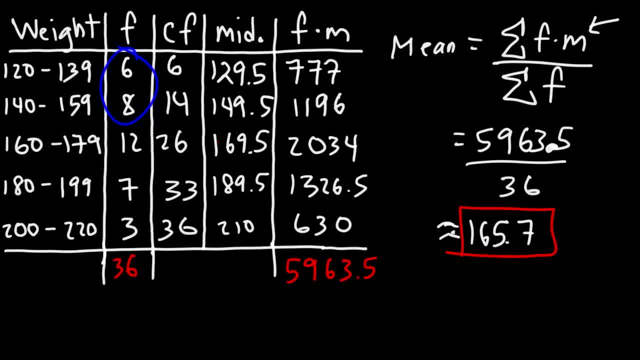 So the median is basically the interval with the highest frequency, which is this one again: 160 to 179.. Now the median half of 36 is 18.. Keep in mind, 36 is the number of students that we're measuring the weight of. 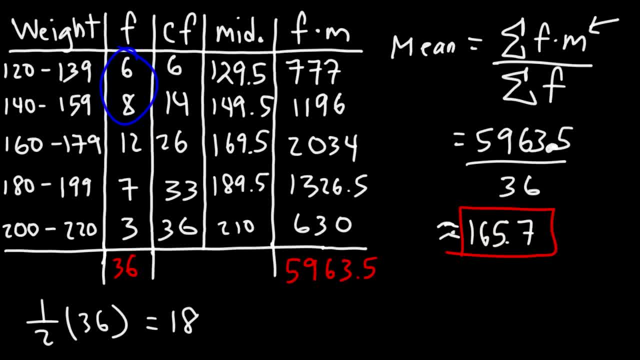 So half of that is 18.. And which interval is the 18th student located in? Now this interval is for the first six students. So if we were to write a range, it will be from 0 to 6, or technically, from 1 to 6.. 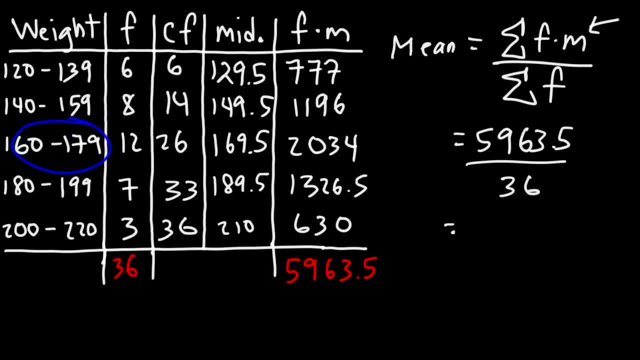 Now most of the numbers are between 160 and 179. And the left side of the data is heavier than the right side of the data, So it's either going to be in this interval or in this interval, one of those two. 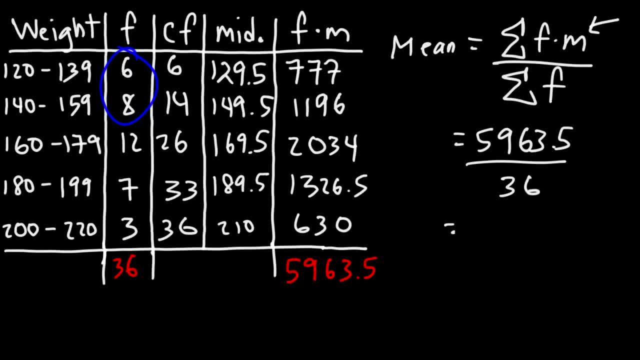 So if we take 5963.5 divided by 36,, that's going to give us 165.7 approximately. So that's the mean which turns out to be in this interval, But notice that it's closer to 160 than it is to 179. 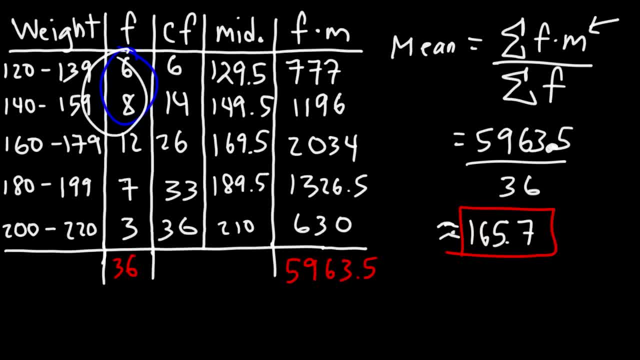 And this is due to the fact that the left side of the data is heavier than the right side of the data. Now, which interval contains the median and the mode. So the mode is basically the interval with the highest frequency, which is this one again. 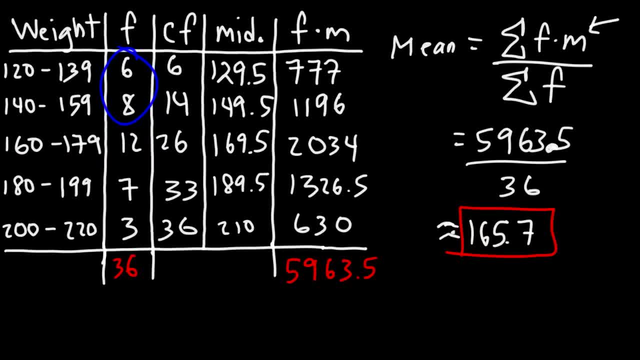 160 to 179.. Now the median half of 36 is 18.. Keep in mind, 36 is the number of students that we're measuring the weight of. So half of that is 18.. And which interval is the 18th student located in? 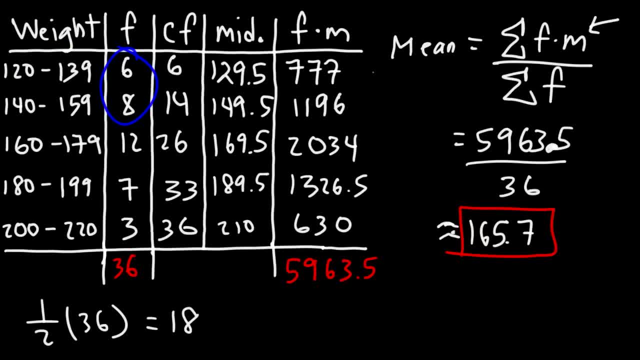 Now, this interval is for the first 6 students. So if we were to write a range, it would be from 0 to 6, or technically, from 1 to 6.. Now this range or that interval covers a range of. 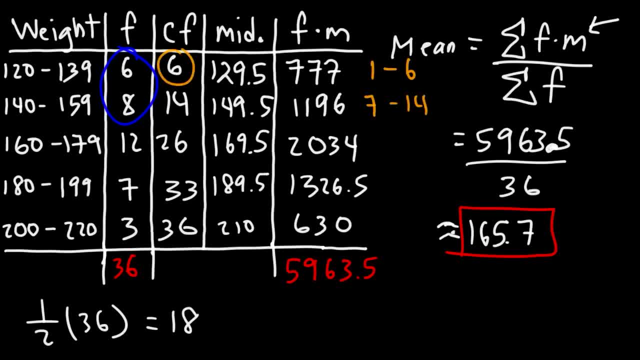 7 to 14.. You start with the next number and you stop here. Now the interval from 160 to 179, it starts from 15 and it ends in 26.. So 18 is in this interval, which means that the median is also located in this interval as well.